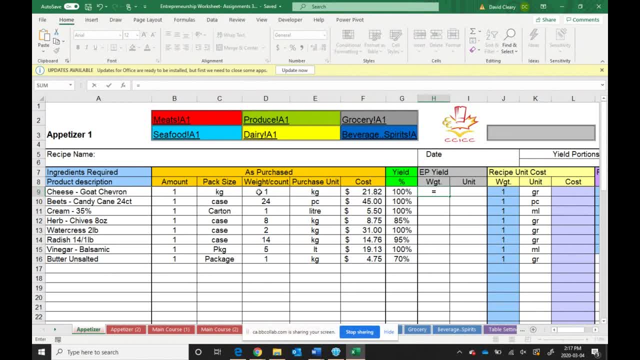 So how we calculate our edible portion yield is by taking the amount in the pack and then multiplying it by the yield. Okay, so let's get one. One multiplied by 100 is one, Or more specifically, in this case it is one kg. 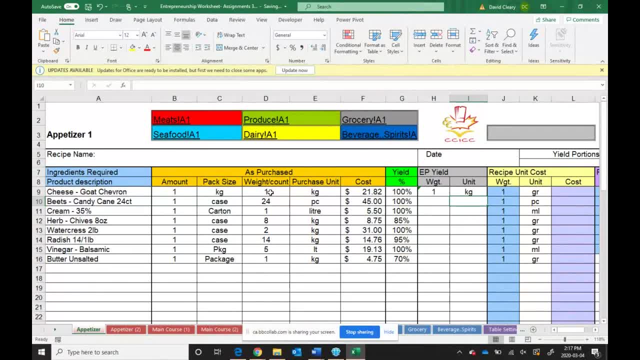 The majority and it depends on where you've got your costing information, but if you've got your costing information from the database that I had posted, the majority of the weight or count for each product is normally going to be one. So one kg, one piece, one litre, one kg and so on. 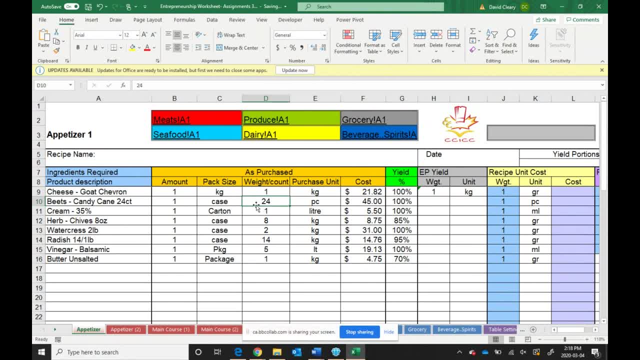 If you've got it somewhere else, you and the pack includes more than one unit of measure, then you're going to have to include them here, okay, Okay, So with that we're just multiplying across. So we have 24 beets that have a yield of 100%. 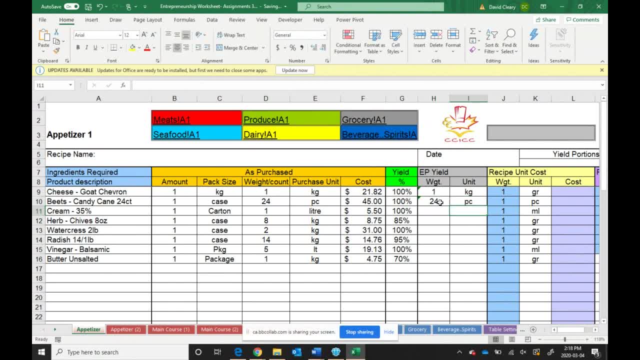 We get 24 pieces. okay, The only times I'm just going to do this quickly here so I can show you there we go, the only times where we're going to have less than we actually purchased, oops- is when there's. 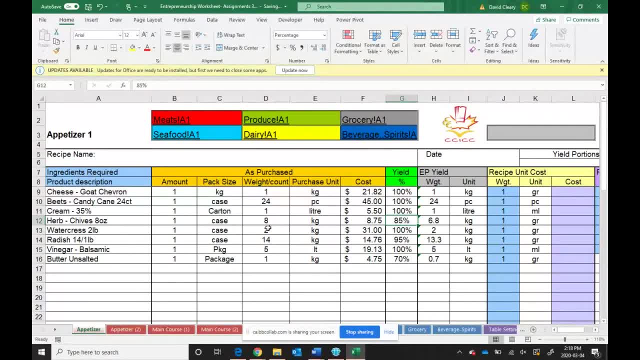 a yield less than 100%. For example, here are chives. We started off with eight kilograms of them Because they have an 85% yield. when we take into consideration the yield, we really only have 6.8 kgs. okay. 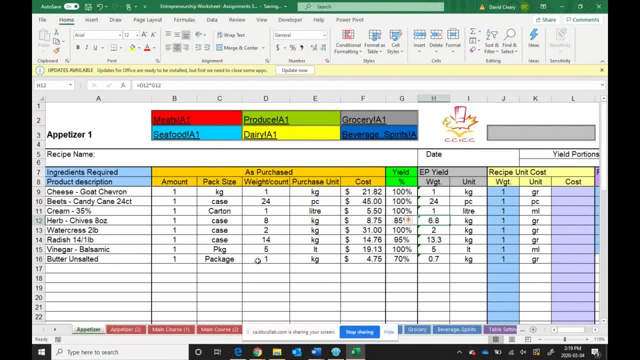 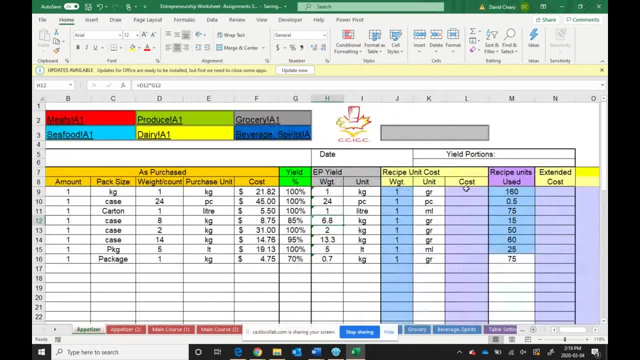 And again, we're calculating that just by multiplying the weight or the count by the yield percentage. okay, As we move across here, we want to calculate essentially the unit cost of each ingredient to be used in the recipe, in the unit that it is used in the recipe. okay, 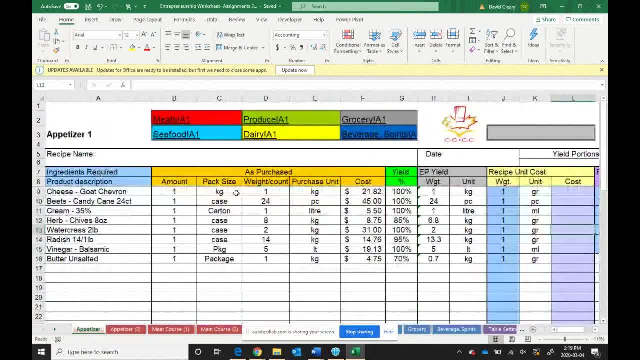 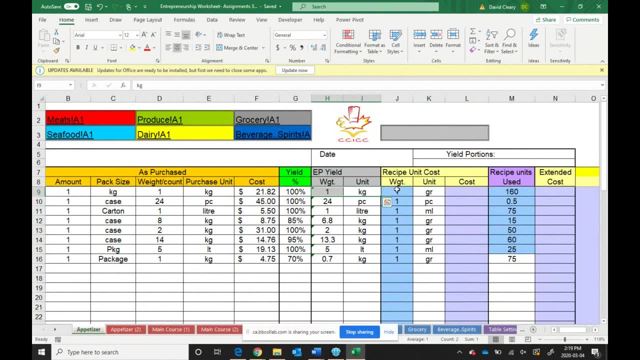 So, for example, here we bought. what is this? This is our goat cheese, So the first line is our goat cheese. We bought goat cheese in one kilogram. However, we're using it in grams in our menu or in our recipe. 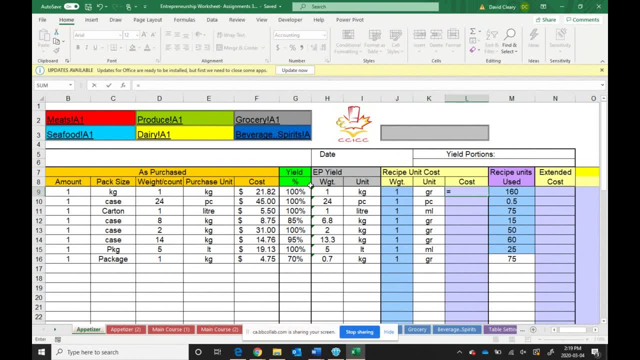 so we have to calculate the cost per gram. So we take the cost per kg and then divide it by 1,000, because there are 1,000 grams in one kg. Next we have the cost of whatever these were. 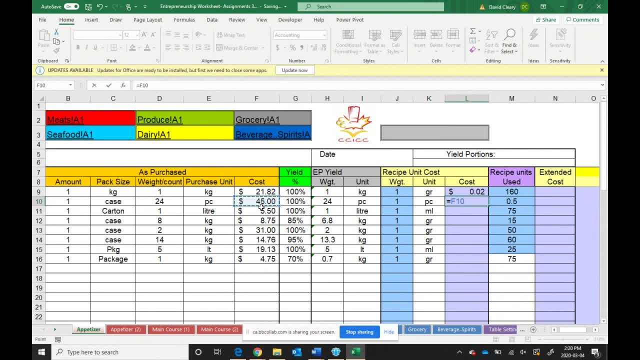 It cost us $45,- what's it called $45, and $24 came in. So we did math: We get $1.88 per piece. okay, Same thing here: Millilitres. we take the cost of the product and then divide it. 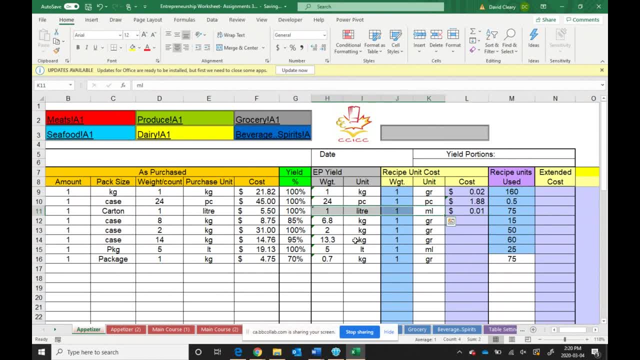 by 1,000, because there are 1,000 millilitres in one litre. okay, Now here's where it gets a bit tricky. okay, It's when products have a yield less than 100%. okay, To illustrate, we started off with eight kgs, when we take into 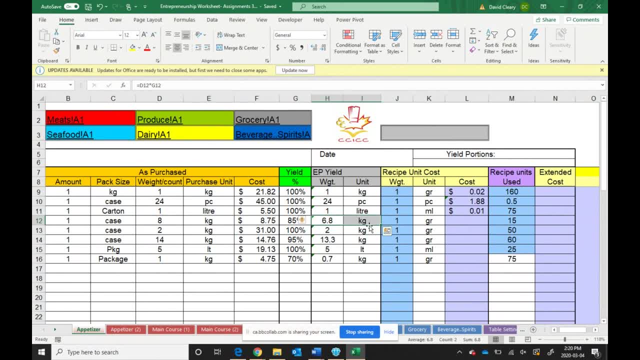 consideration the yield, We only have 6.8 kgs. okay, So the cost per kilogram is going to go up. We need to show that and take that into consideration when we're calculating the cost per one gram, And I'll show you how to do that. 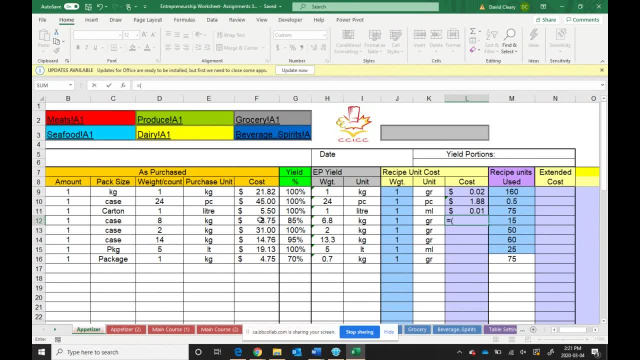 So what we do here is take our the original cost. in this case it was $8.75.. We're then going to divide it by the edible portion And remember it has a yield of 85%, so less than 100. 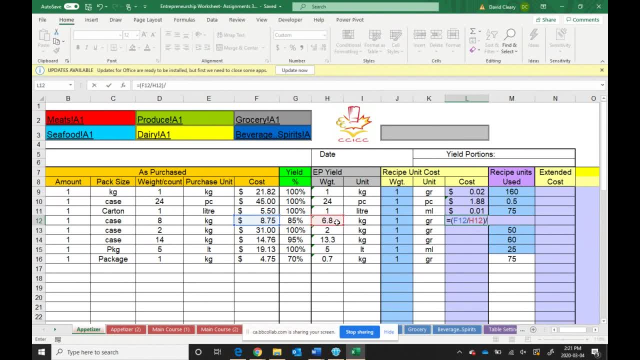 We're then going to, after we've done that math, we're then going to divide that by 1,000, okay, Here the next one. we had 100% yield. so the math is super quick, okay? Actually no, because it came in a pack of two. 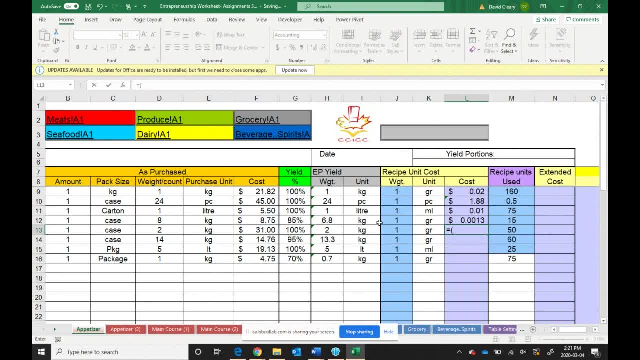 So we have to take this: take the original cost, divide it by two kgs to get the cost per kg. There we go, And then divide it by 1,000 to get the cost per gram. okay, Here another complex one, because it has a yield less than 95%. okay. 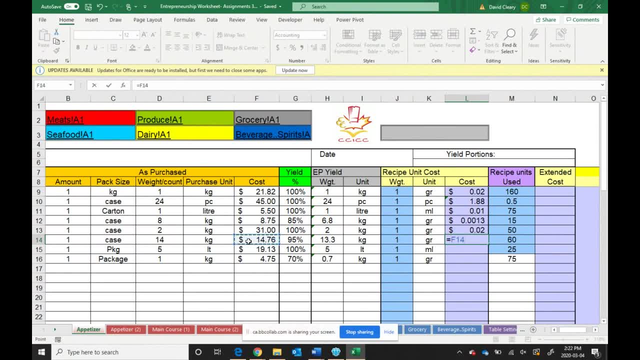 So we take the cost. sorry, I'm going to put the bracket around it. We take the cost. we then divide it by the amount of kgs that it actually yielded, okay, and then we divide it by 1,000, okay. 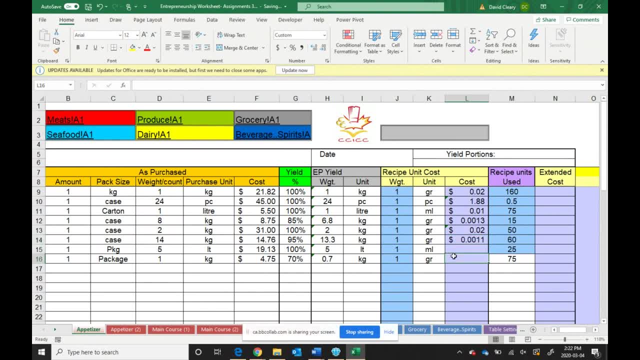 Make this a bit bigger here. There we go. Okay, Here we have a product that had more than one unit measure. So we take the take, keep forgetting the brackets. Take the cost, divide it by the amount of the product in the. 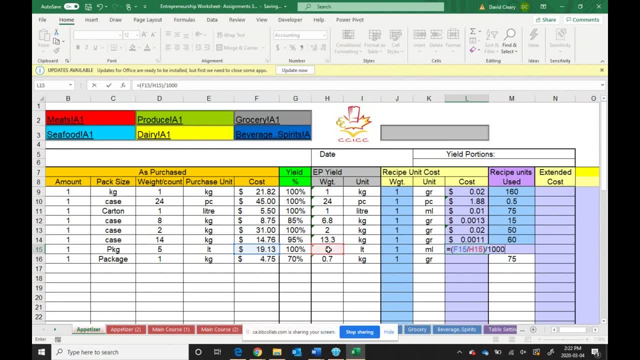 pack like that and then divide it by 1,000, because there are 1,000 millilitres in one litre. So there we are, Okay, And then here's another yield that has less than 100%. So we take the cost, take the cost, divide it by the amount of. 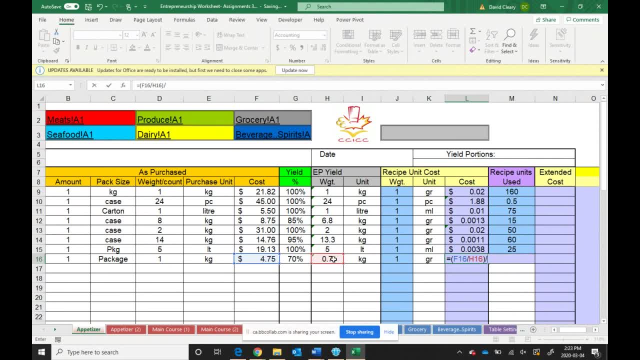 the product in the pack, close the bracket and then divide it by 1,000, because there are 1,000 grams in a kilogram. So now that we've done that, these are the unit costs, or unit costs that we're going to be using to cost out the amount of 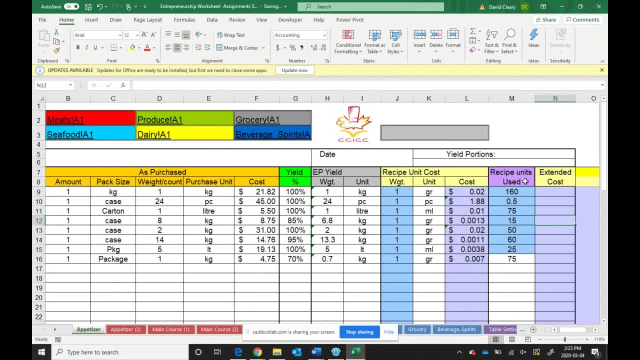 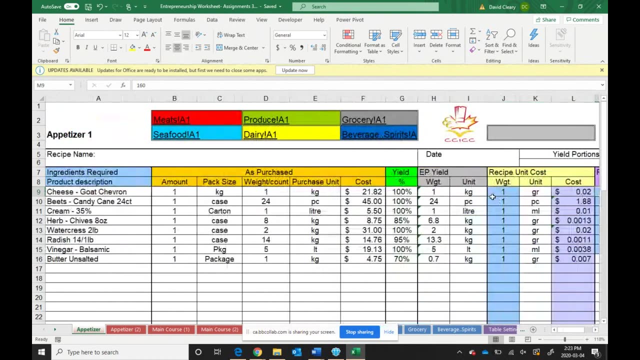 product in the recipe. okay, So the next step is to calculate our extended cost. Important to note here the recipe units used is the amount of each product used in the recipe. For example, here our goat cheese, we use 160 grams of goat. 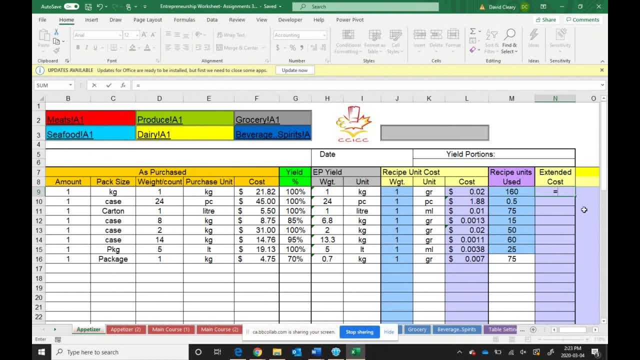 cheese in this recipe. So calculating the extended cost is quite simple. We take the amount of the product in the recipe and then multiply it by the unit cost. There we go. A really easy way to do the rest of this. well, I'll give you. 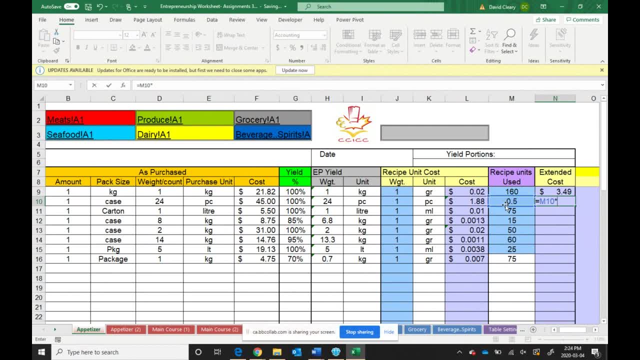 another example before I show you that. So we're taking the amount of the product in the recipe and multiplying it by the cost. There we are, And if you wanted to calculate the formula and drag it, if you wanted to copy the formula to all the cells below, you would do this. 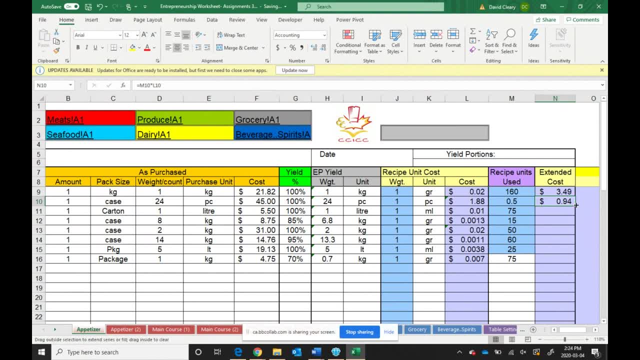 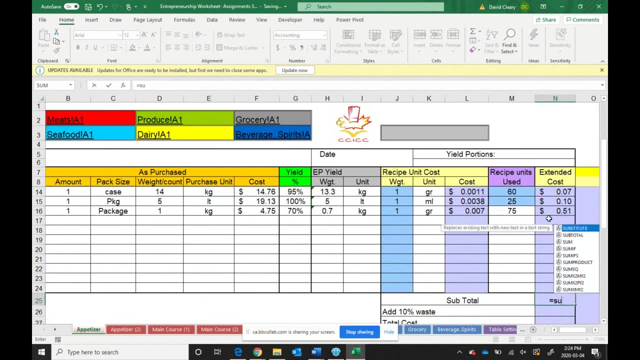 You just grab the little blue or green box on the right-hand side, click it and drag it all the way down. there you have it. We have all of our extended costs. So if I go down here I want to add up all of those extended.